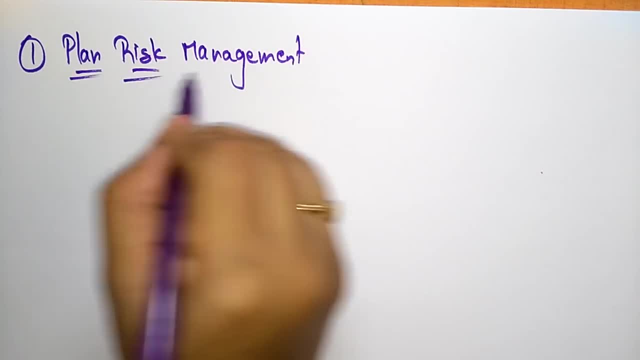 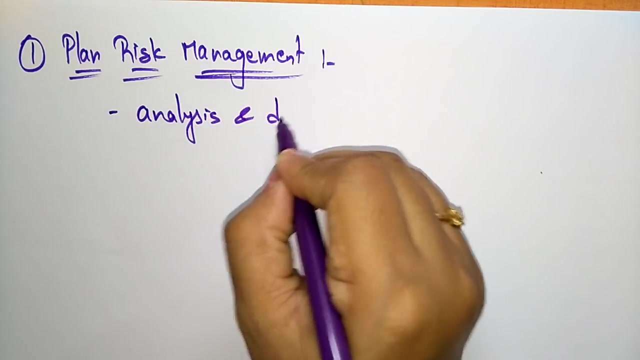 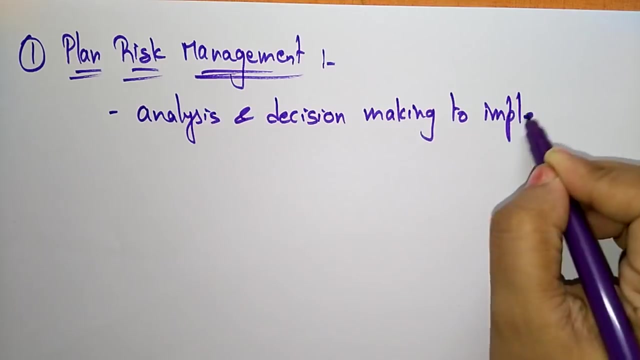 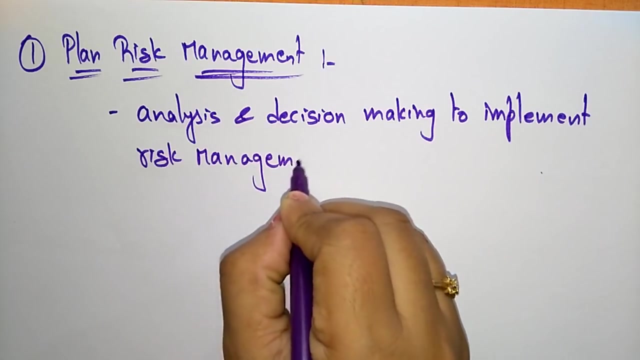 The plant risk management. it is going to be analysis and decision-making to implement risk management. the first thing it is: it is an analysis, analyzing and decision making. make you two, you two implement to implement risk management. so, the first thing, the plan. if you want to plan the risk management, what are the risks that are involved in the project? 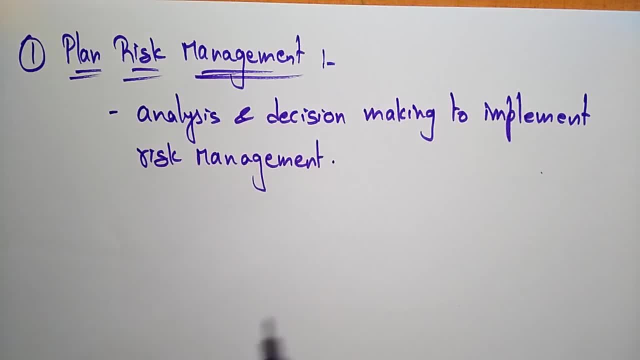 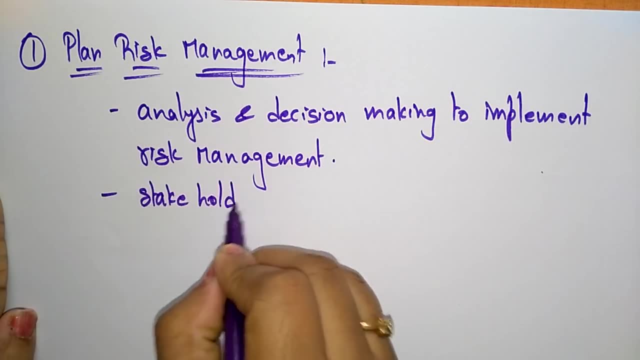 first you have to analysis the project and you have to make some decision to implement the risk management. so next the stockholders will be there. the person who is going to be affected if you are implementing the project means the person. he's maybe a manager, he is maybe a customer, he's anything. the 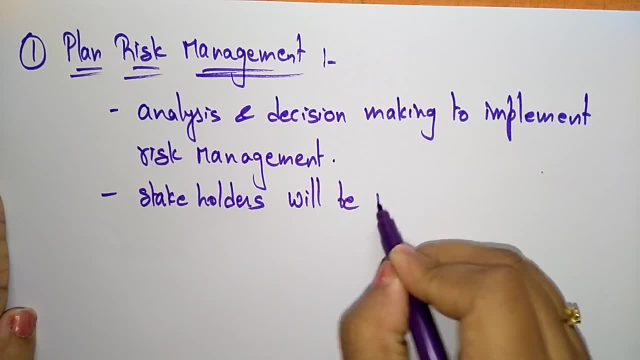 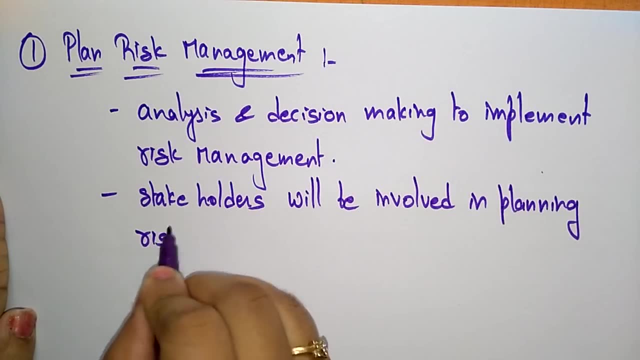 stockholders will be involved in planning risk management because they are going to be affected if anything. if risk, that may be a positive or a negative impact, that impact will be has to be fazed by the stockholders also. so we have to be involved those stockholders also in the planning of 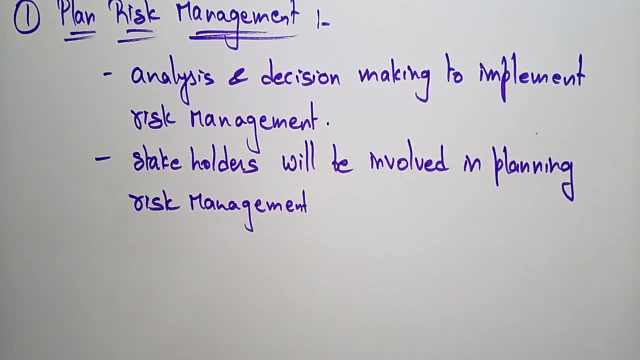 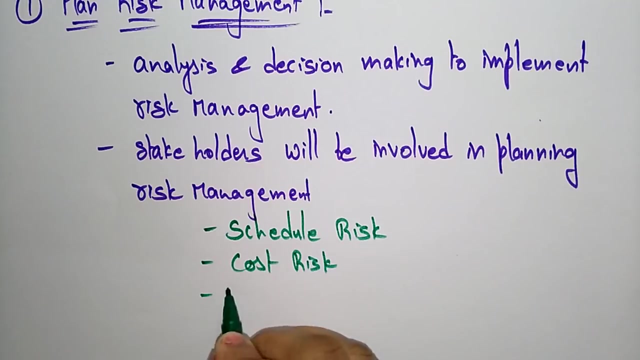 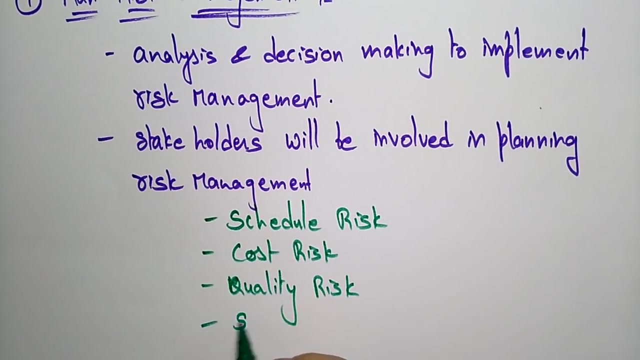 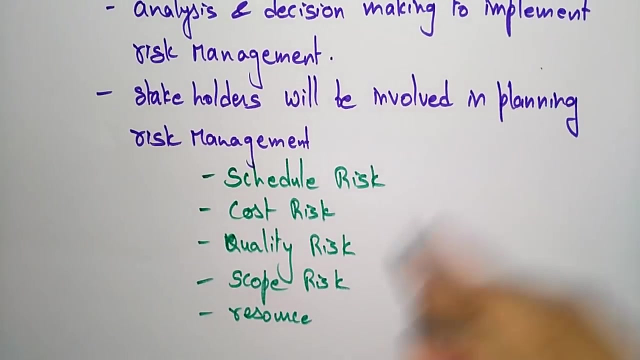 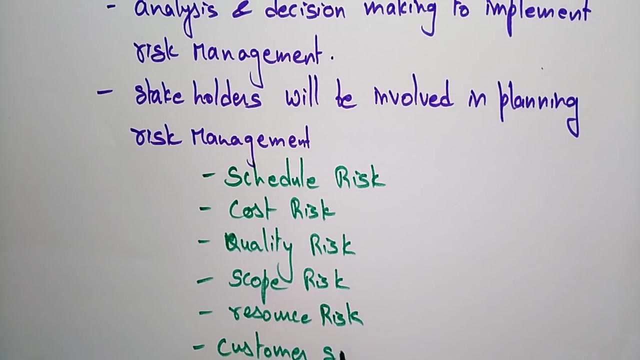 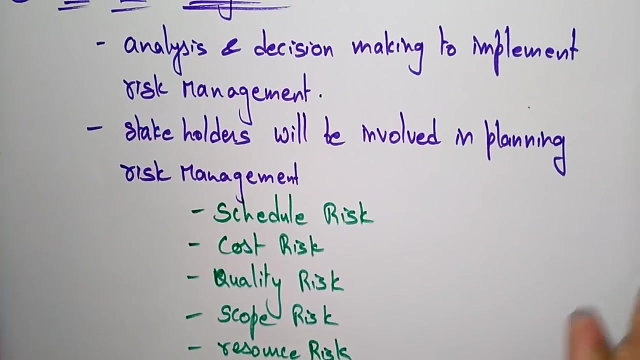 risk management. risk management so the different risk that may be affected by the stack holders or any of the organization or the customer or the software engineering or schedule risk, schedule risk, cost risk, quality risk, scope risk, resource risk, resource risk, customer satisfaction risk, customer satisfaction risk. so if you want to plan the risk management, 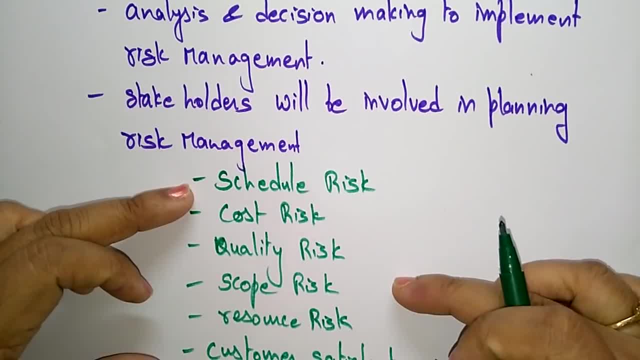 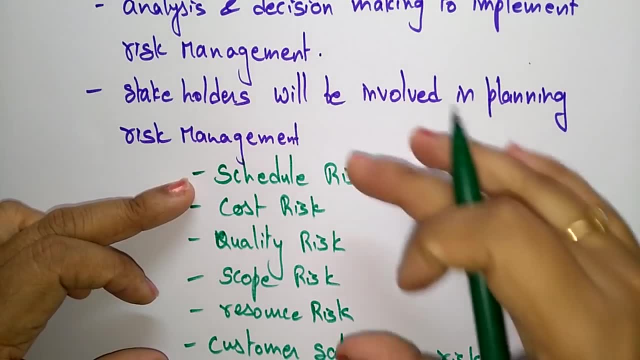 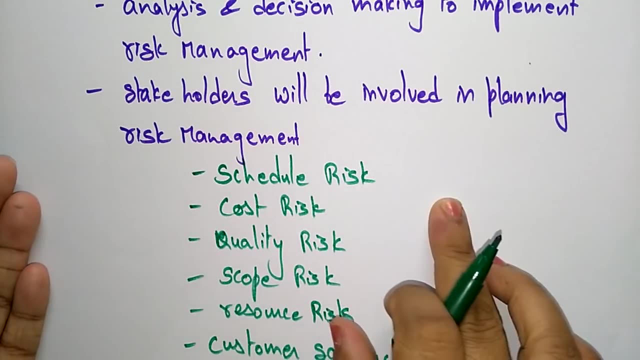 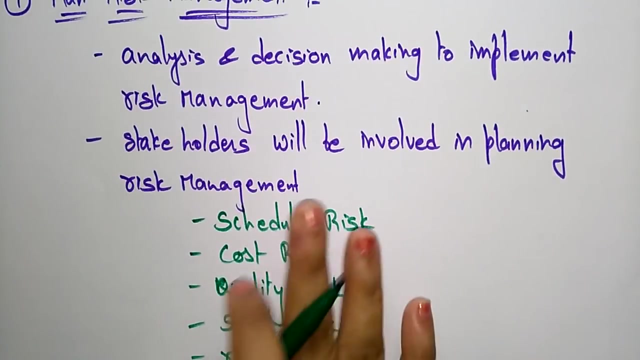 you have to take care about these risks that are involved while the planning the project, while planning the risk management, not the project, the while planning the risk management. so these are the quantities you have to be take care about planning the risk management. they have to schedule risk, cost, quality risk scope, risk, resources and customer satisfaction risk. so this: 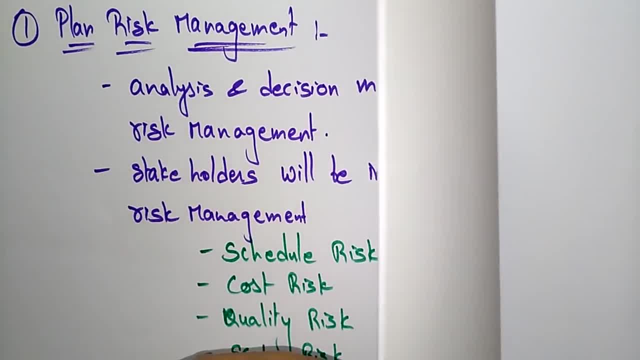 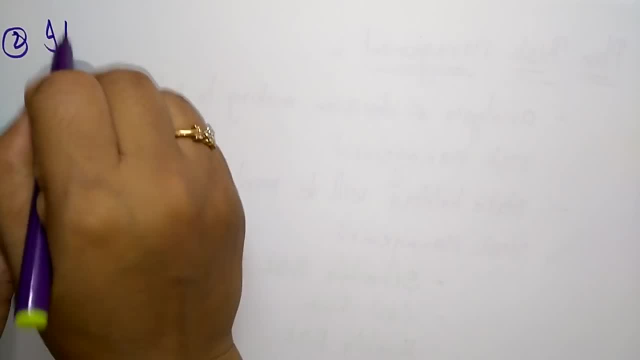 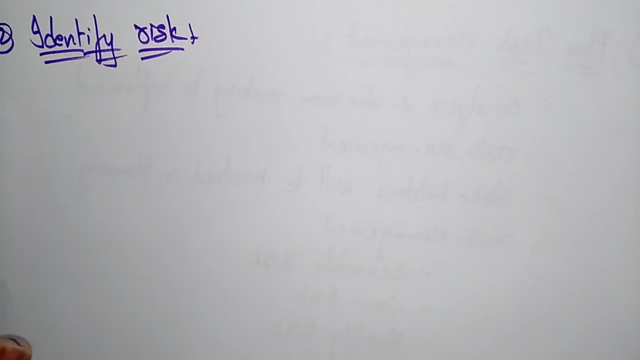 is about the plan risk management. now coming to the next risk in project management is the identify risk. so next is identify risk, so how they are going to identify the risk in the project, so which risk has more probability of affecting the project that we have to be identify first. so while dealing with the risk management, 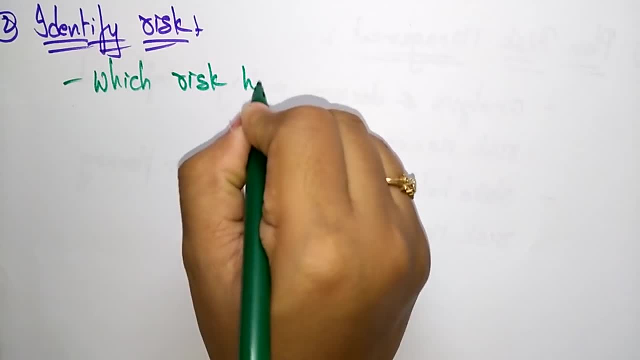 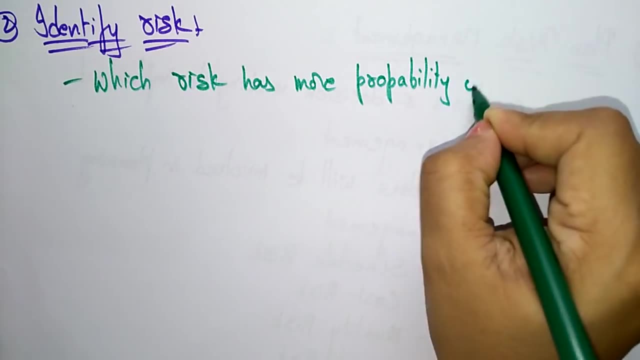 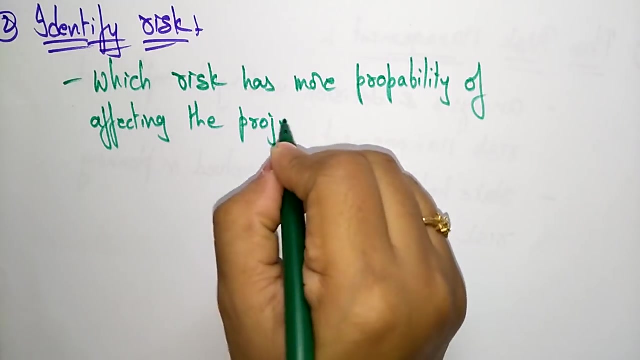 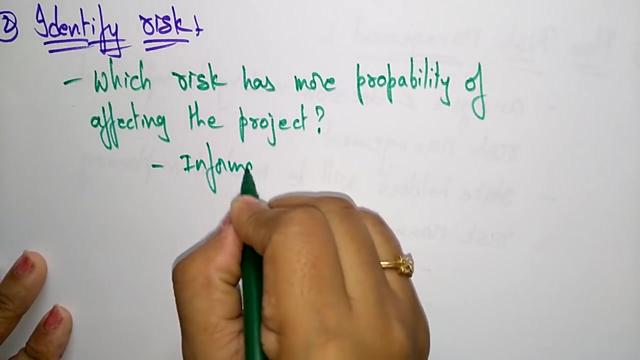 they have to be check which risk has more probability, more probability of affecting the project. so which one is affecting the project we have to be check. so that is the one way of identifying the risk. so the information gathering checklist- and also how you are going to be after identifying this risk. the information has to be gathered. information gathering checklist. 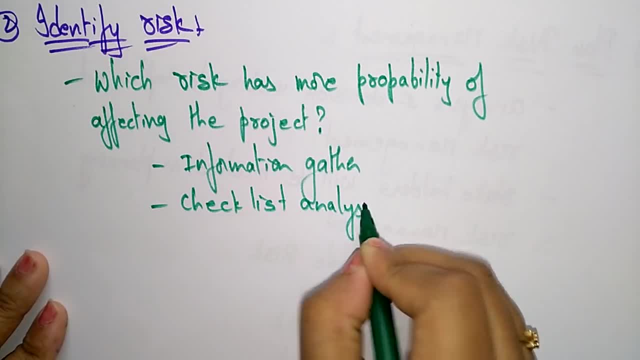 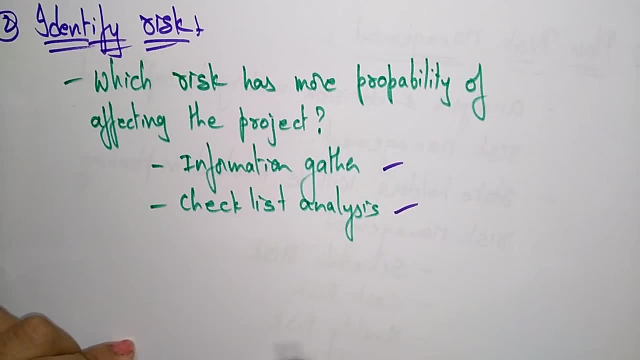 analysis. what are? what are these two actually? with the help of the information gathered, you are going to be identify the risk and with the help of the checklist analysis, you are identifying the risk means before starting the project at the time of uh requirements, you have to make the uh project. 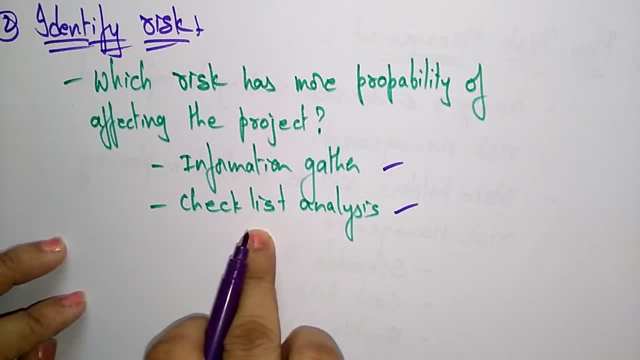 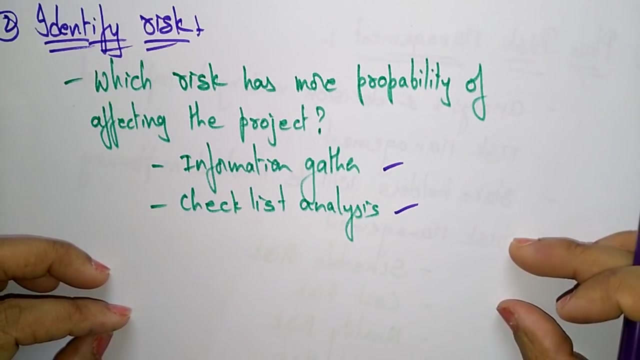 means the requirements in an order. means you have to make a checklist, the checklist analysis. if you make checklist, uh, while doing the project means first i have to start this. okay, i complete after the completion of the phase, this phase. i am going to start this phase after the completion of this. 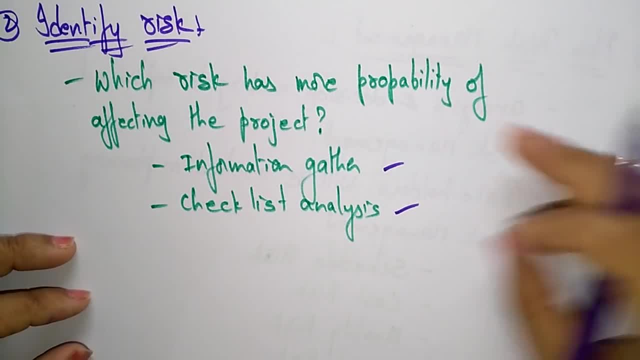 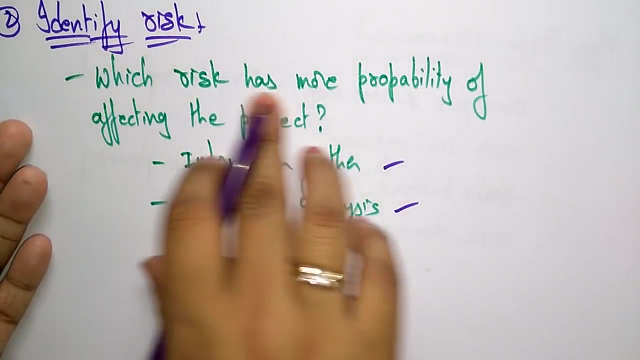 phase, i will go for the next phase. so you have to be make a checklist so that, uh, if there is any uh risk that is present in the each phase, that can be identified easily. so this is a way you can identify the risk. so first you have to take about which risk has. 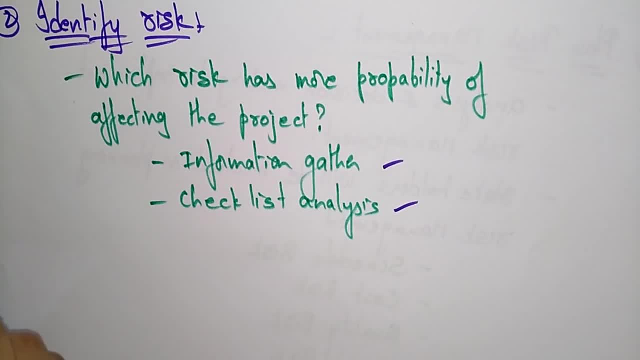 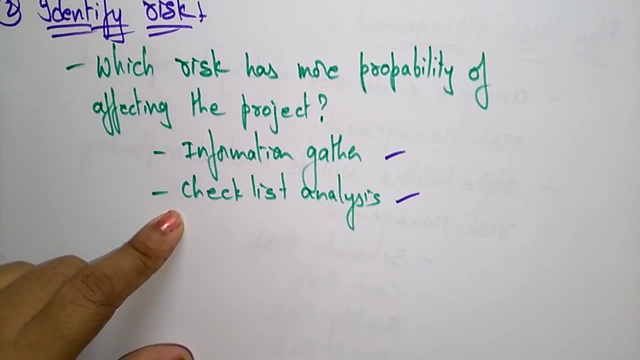 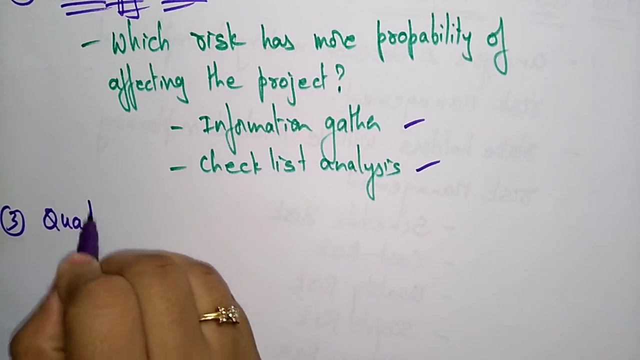 more probability of affecting the project. so that can you can be identified. so next, you can identify it by using the information gathering or by using the checklist analysis. okay, now coming to the third one. what is the third one? the third one is the qualitative risk analysis. qualitative means a quality product. if you want to make a quality product, so in for in developing the 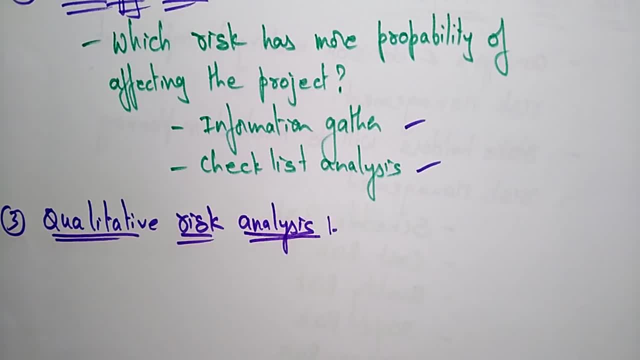 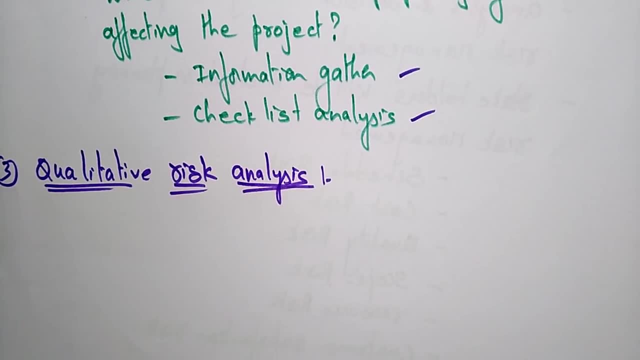 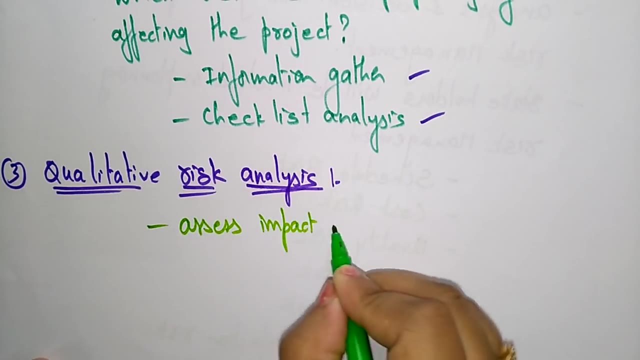 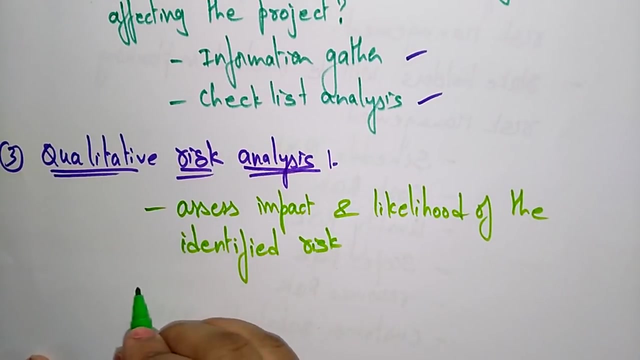 quality product also if some risk will be available. so what are the qualitative risk analysis? the first thing is ss impact. it is going to be ss impact and likelihood of the identified risk, of the identified risk. so next, the risk management assessment with the help of risk, not risk urgency assessment. 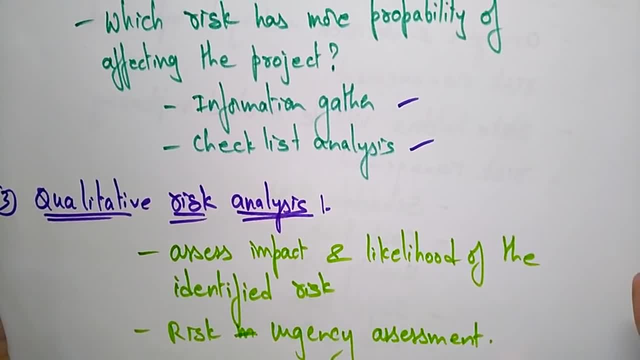 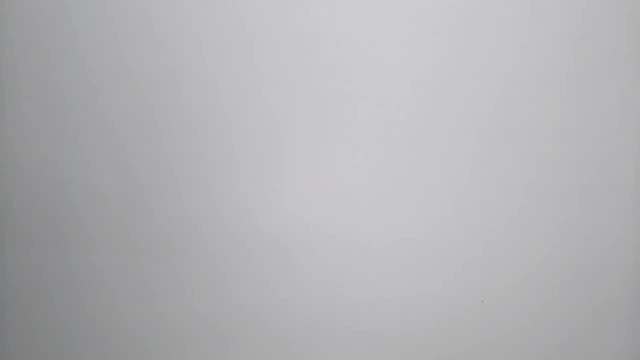 so this is about the qualitative risk analysis. so if the risk management is going to be 60%, that is a risk, scared of it. still, you are having the three risk uh in project management. let's continue with the fourth one. what is the fourth one? the fourth one is quantitative risk response: risk analysis. 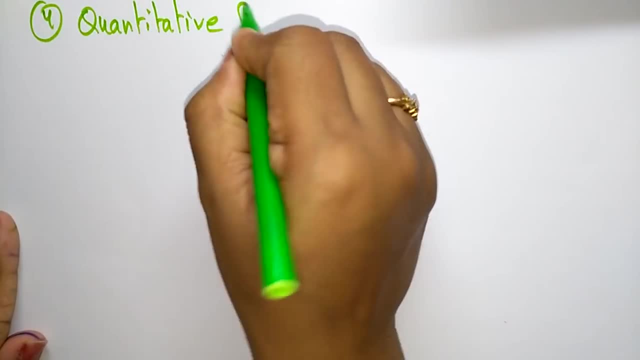 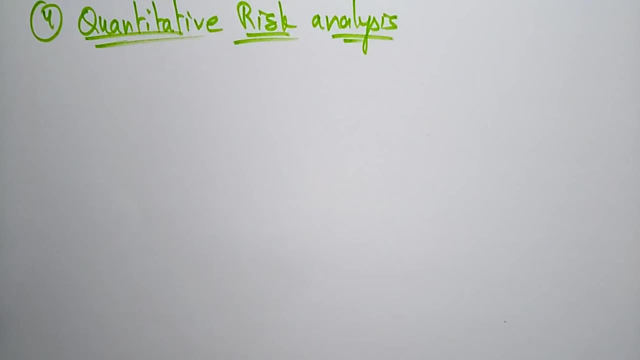 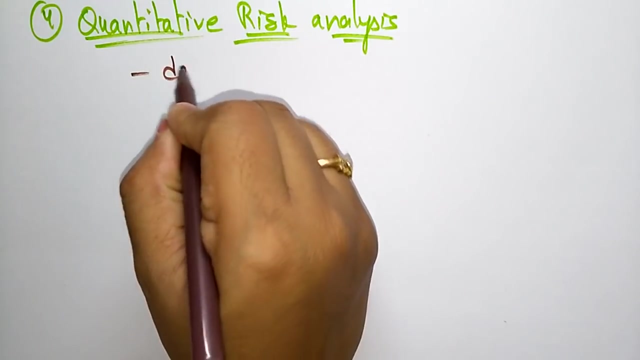 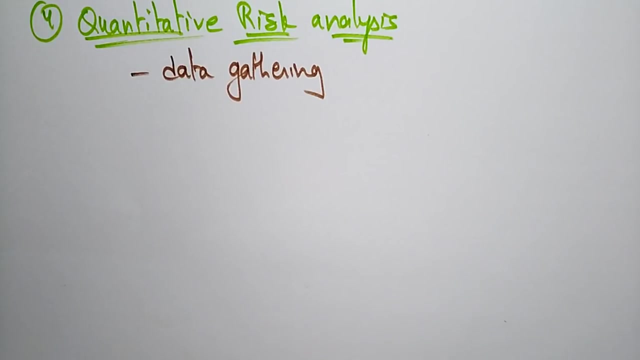 quantitative risk analysis. so in the previous uh i explained the third one is the qualitative risk analysis. now it is a quantitative risk analysis. the quantitative risk analysis can be identified by data gathering. data gathering, so how much data that will be there to develop a project that is a? 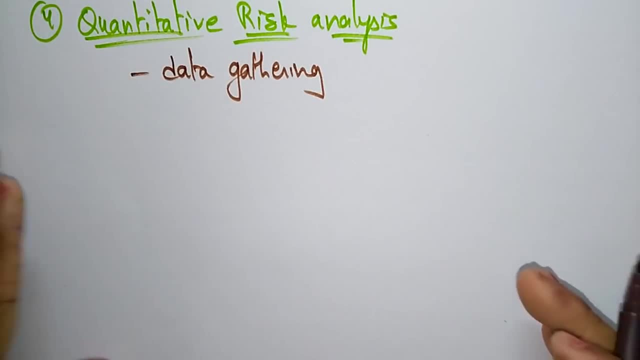 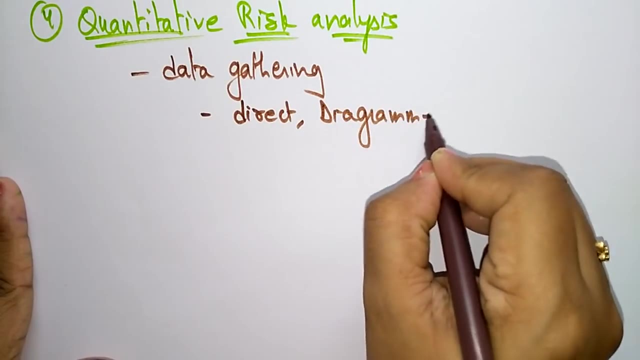 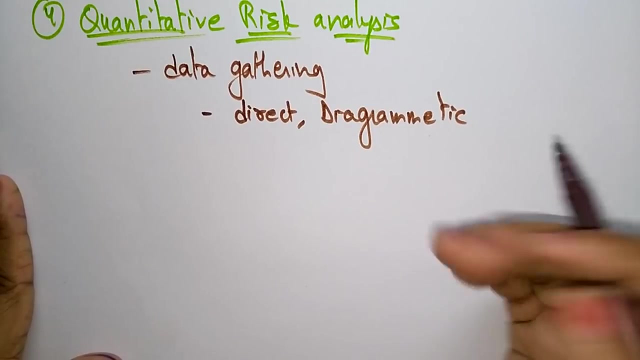 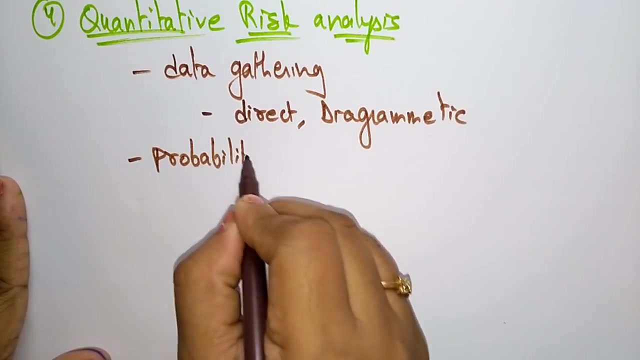 quantitative means measuring, okay, the data gathering. that you can be done by direct or diagrammatic. with the help of diagrammatic, using the some diagrams, umls diagrams- you can measure the quantitative risk analysis. or you can measure directly and probability distribution, probability distribution, next, modeling techniques. so with the help of this, you can, uh, measure the quantitative risk. 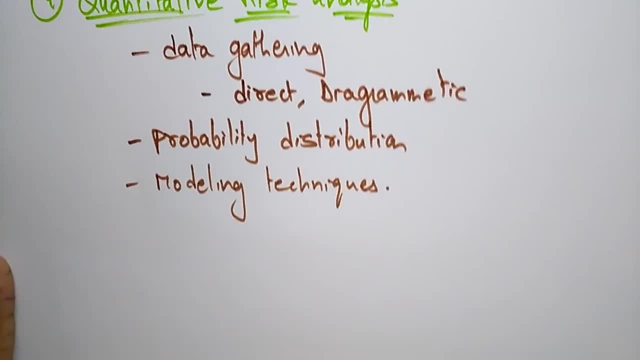 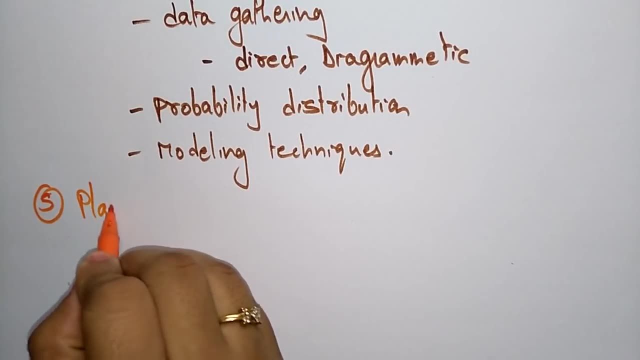 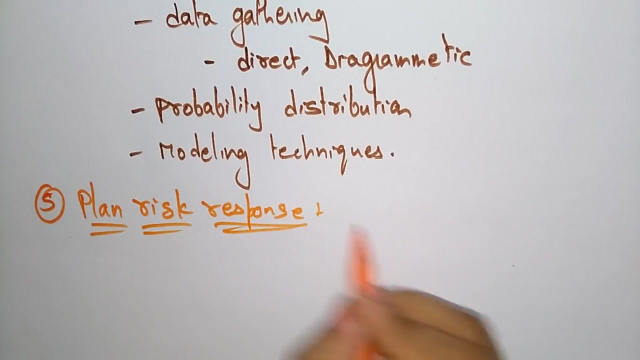 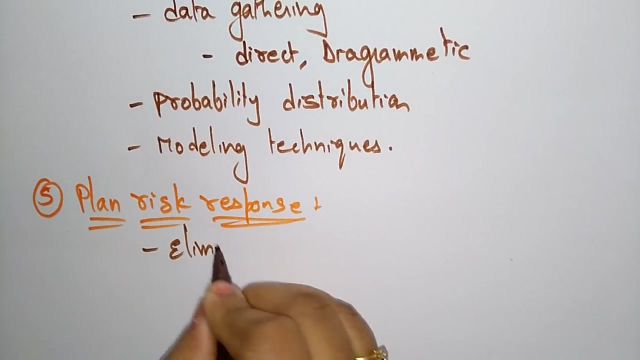 analysis that is present in the risk uh project management and the fifth one. so the fifth one is plan risk response. plan risk response- how it is going to be. response: the plan dress crespon. the plan risk response: first, it eliminates the threats. eliminate threats before they happen. so, starting before starting on, only you have to try to eliminate the threats. 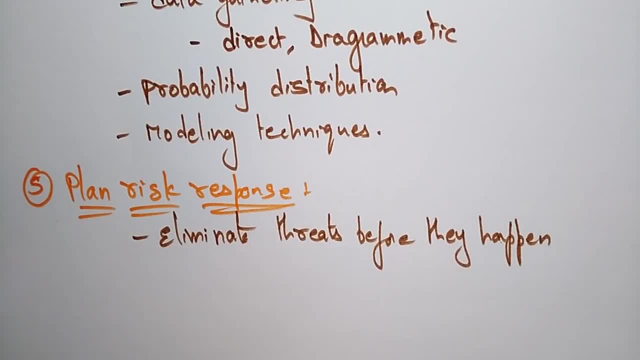 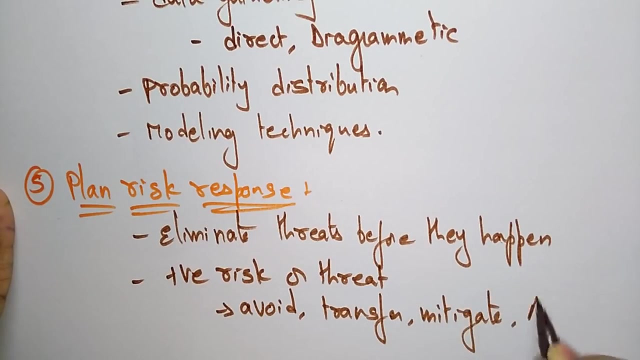 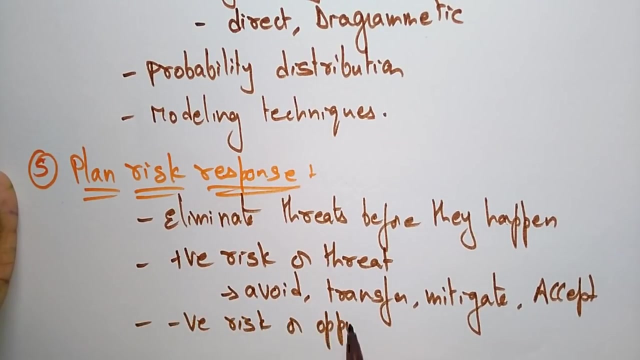 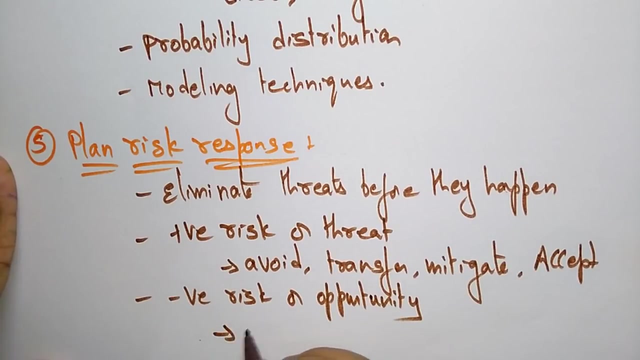 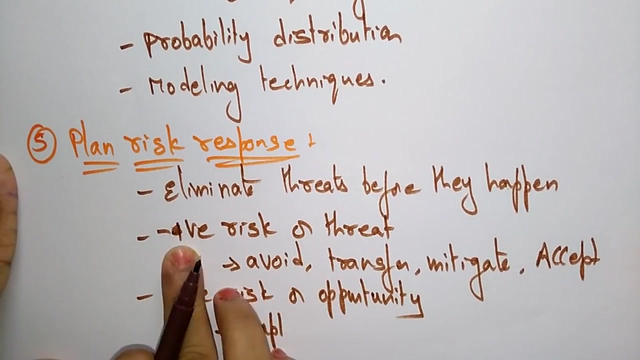 So that it decrease the impact of threat. Next, the positive risk or threat. So in the planned risk analysis if there is a positive risk or a threat is occurred, then it can be: avoid, transfer, mitigate, after that accept. Next, suppose it is a negative risk or opportunity is observed, You have to be exploit. Sorry, this is a negative risk and this is a positive risk. Negative risk or a threat, positive risk or opportunity. 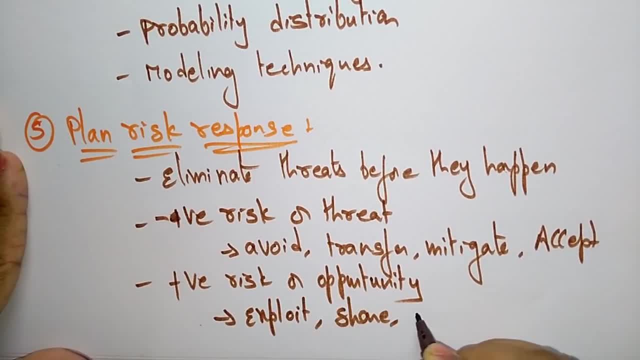 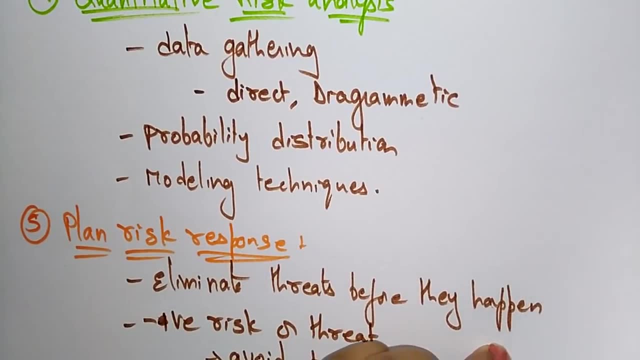 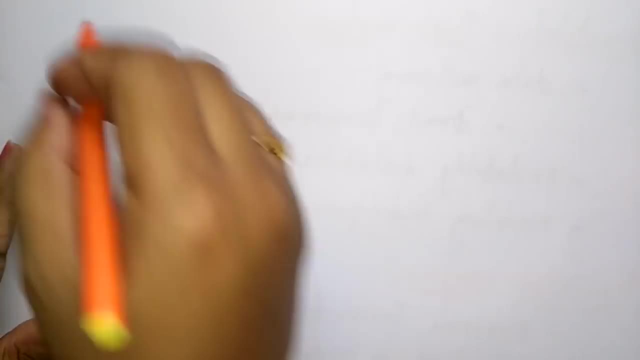 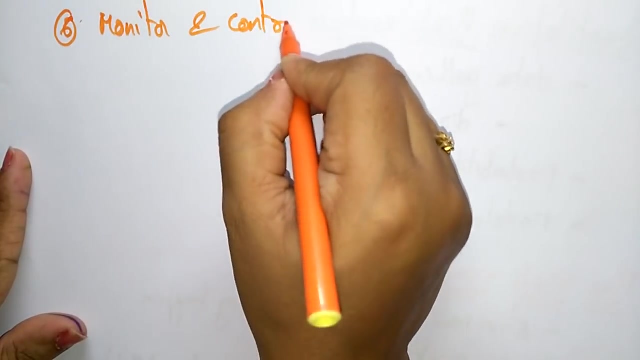 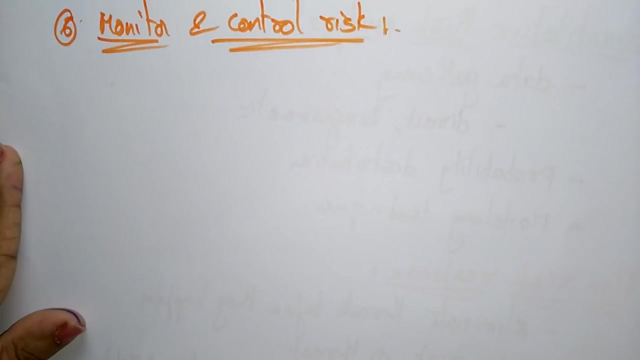 Exploit share enhance. So this is about the fifth one, the planned risk response, And the final, that is a sixth. The sixth one, that is in the risks in project management, is monitor and control risk, Monitor and control risk. So here the risk assessment. 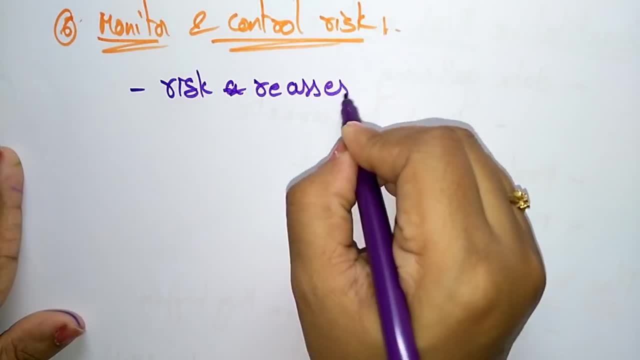 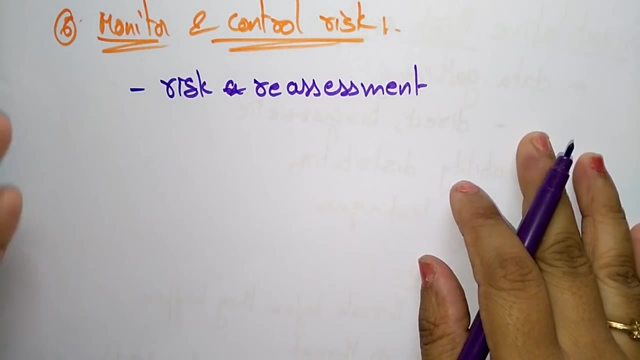 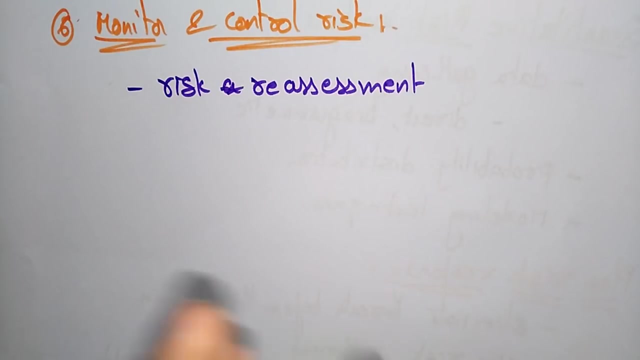 Re-assessment, not assessment. It is reassessment In the monitor and controlling risk. how are you going to monitor and control, that is, with the help of risk? reassessment means the scheduled regularly to identify a new risk. You, you always make some scheduled. 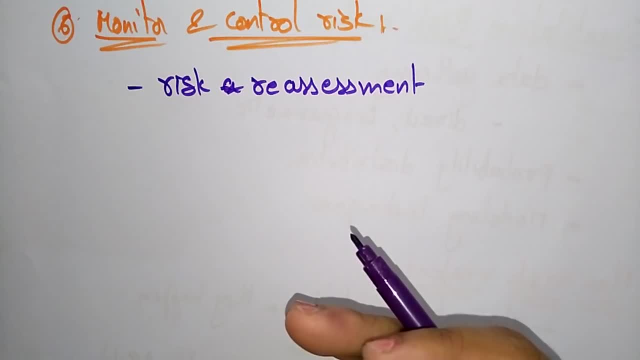 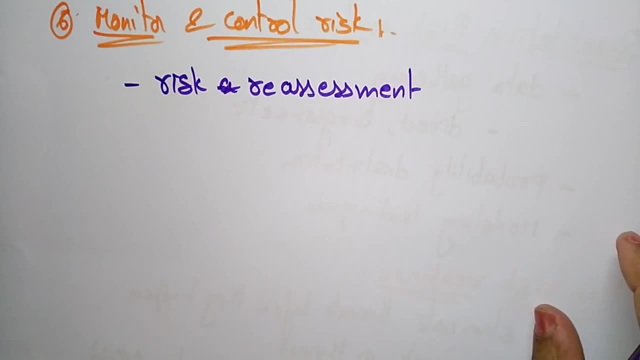 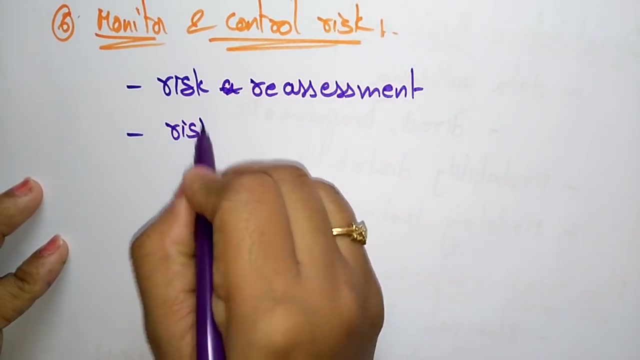 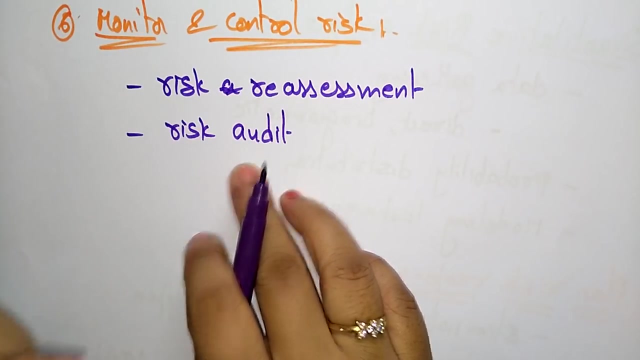 After completion of this, again you have to be scheduled regularly so that you can identify any risks or present in the while you're doing the coding like that, to always monitor by using risk reassessment. next, next risk audit. risk audit means examine the effectiveness of planned risk response. so you have to examine the effectiveness of planned risk.